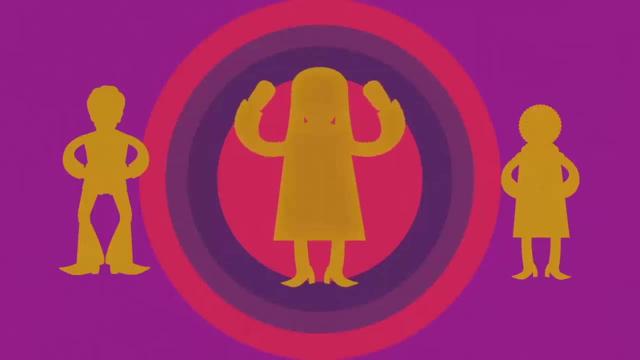 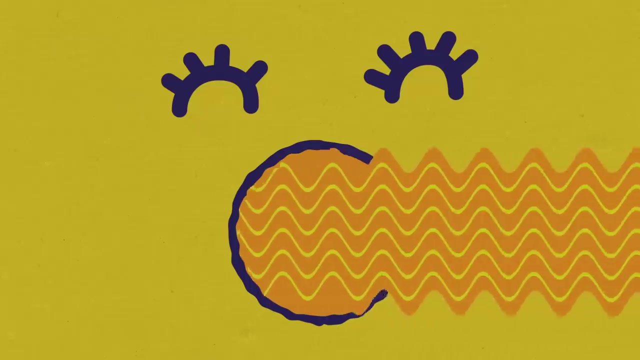 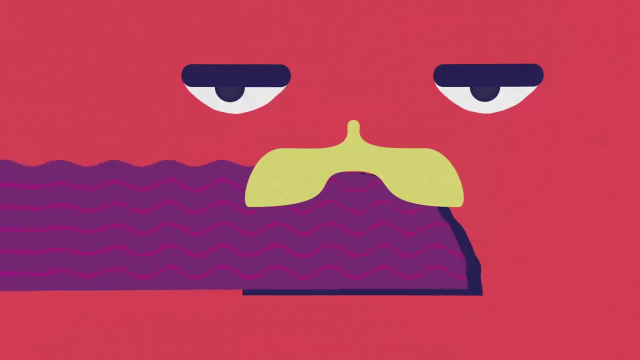 Genes that result in a greater variety of immunities may give offspring a major survival advantage. Our ears also determine attraction. Men prefer females with high-pitched, breathy voices and wide formant spacing, correlated with smaller body size, while women prefer low-pitched voices. 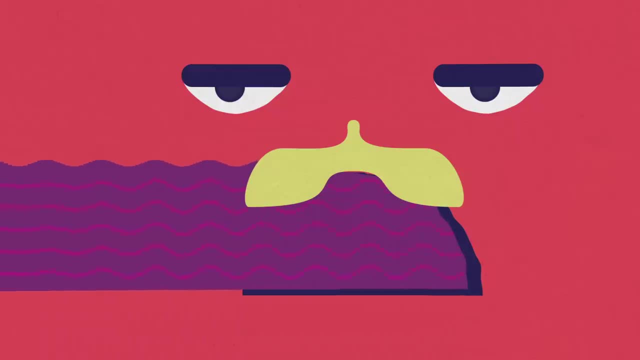 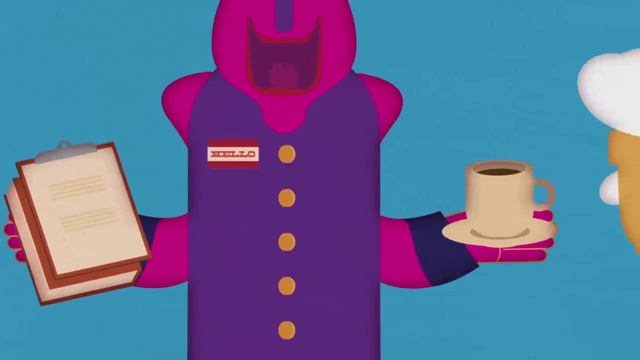 with a narrow formant spacing that suggests a larger body size And, not surprisingly, touch turns out to be crucial for romance. In this experiment, not realizing the study had begun, participants were asked to briefly hold the coffee, either hot or iced. 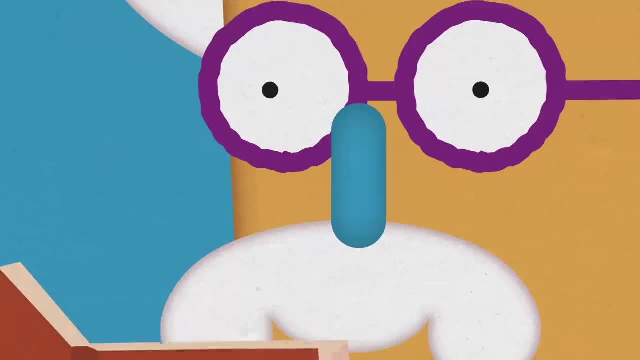 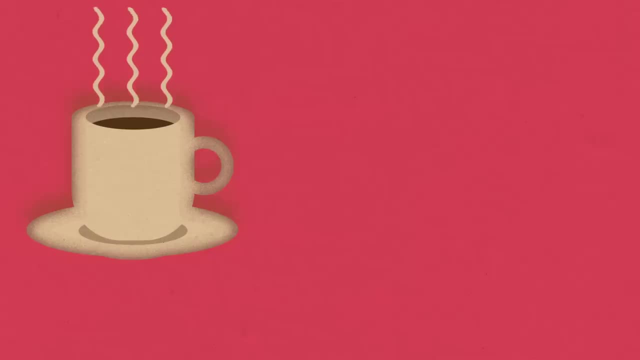 Later, the participants read a story about a hypothetical person and were asked to rate their personality. Those who had held the hot cup of coffee perceived the person in the story as happier, more social, more generous and better natured than those who had held the cup of ice. 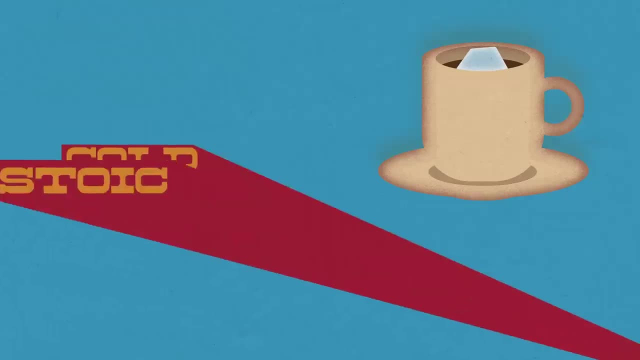 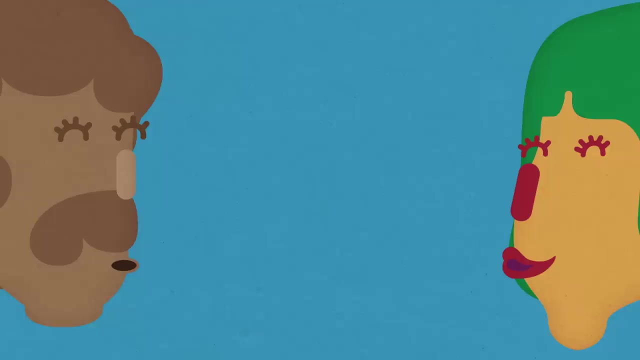 Those who had held the cup of iced coffee, who rated the person as cold, stoic and unaffectionate. If a potential mate has managed to pass all these tests, there's still one more: the infamous first kiss, a rich and complex exchange of tactile and chemical cues. 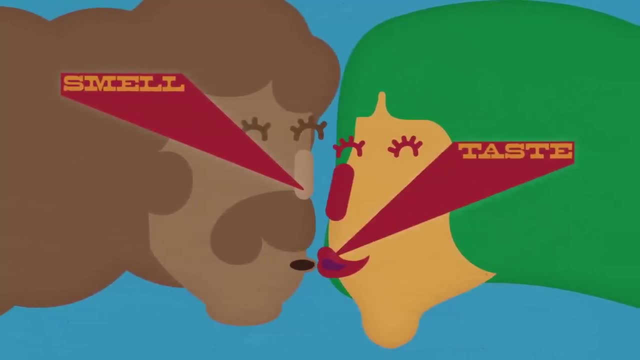 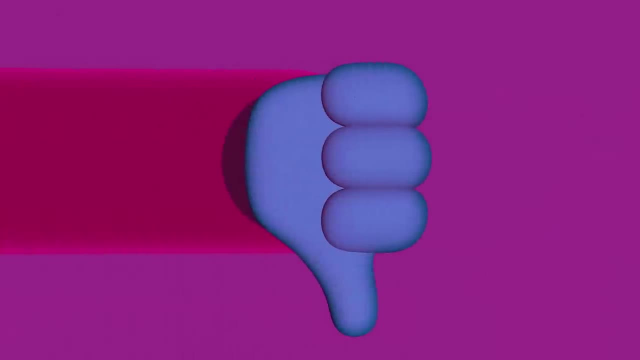 such as the smell of one's breath and the taste of their mouth. This magical moment is so critical that a majority of men and women have reported losing their attraction to someone after a bad first kiss. Once attraction is confirmed, your bloodstream is flooded with norepinephrine. 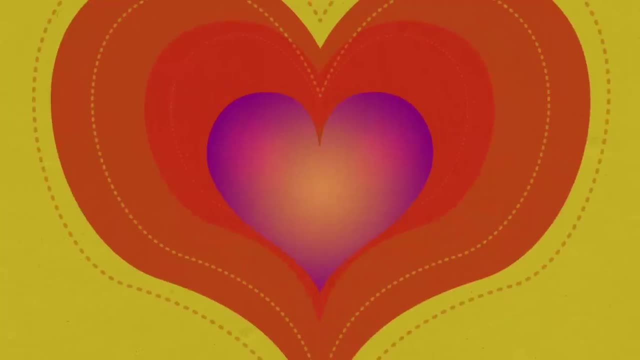 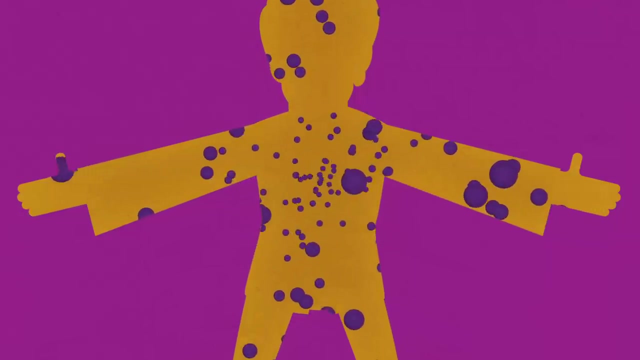 activating your fight or flight system, Your heart beats faster, your pupils dilate and your body releases glucose for additional energy, not because you're in danger, but because your body is telling you that something important is happening To help you focus. 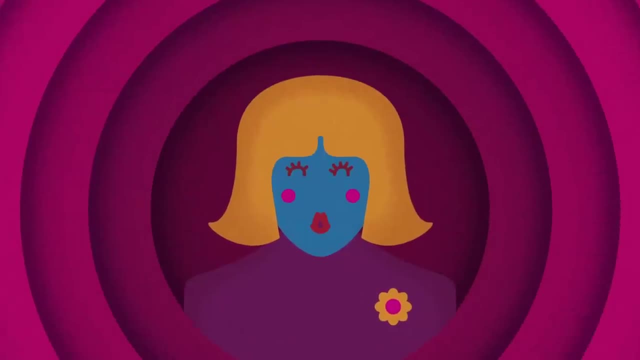 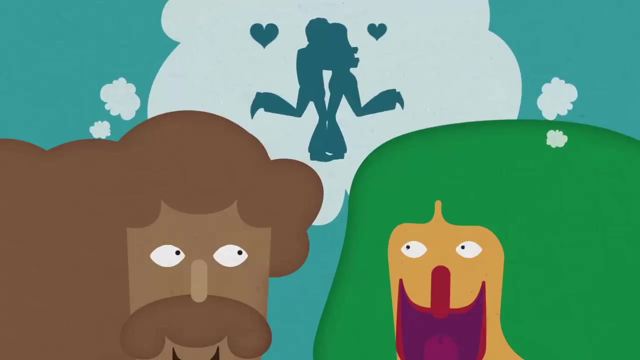 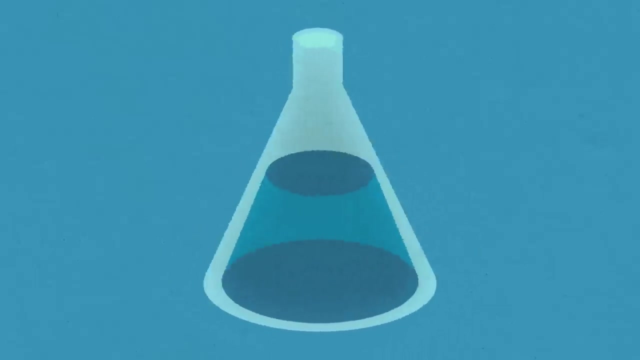 norepinephrine creates a sort of tunnel vision, blocking out surrounding distractions, possibly even warping your sense of time and enhancing your memory. This might explain why people never forget their first kiss. The idea of so much of our attraction being influenced by chemicals and evolutionary biology. 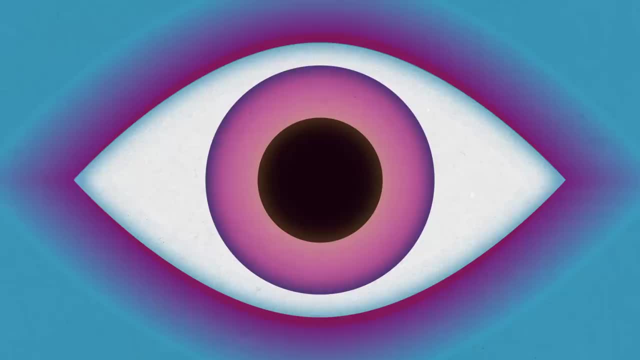 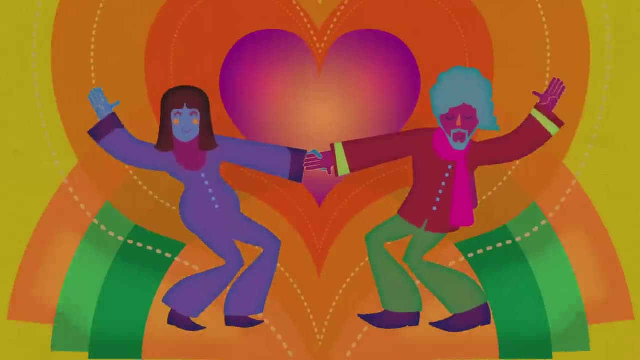 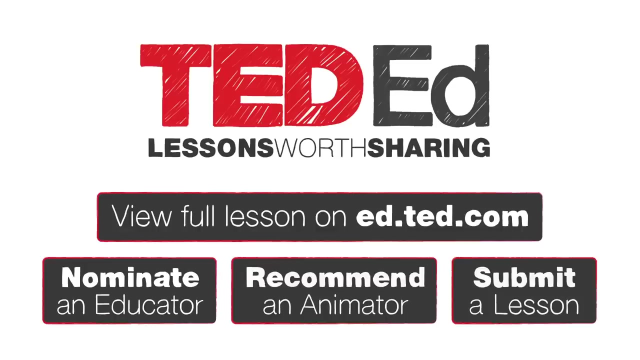 may seem cold and scientific rather than romantic, but the next time you see someone you like, try to appreciate how your entire body is playing matchmaker to decide if that beautiful stranger is right for you. Subtitles by the Amaraorg community.